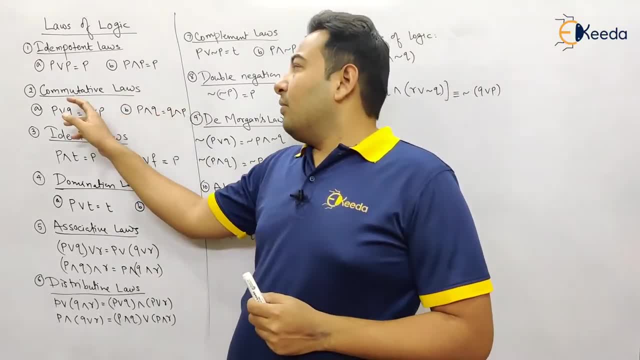 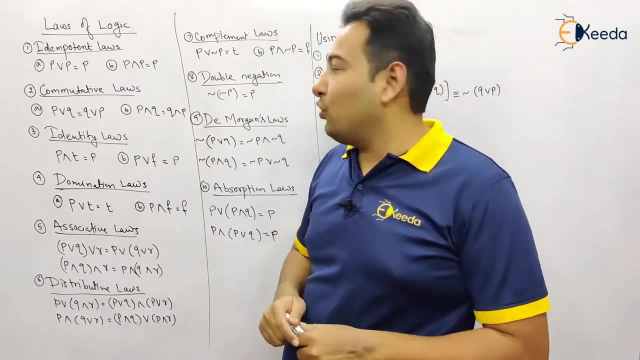 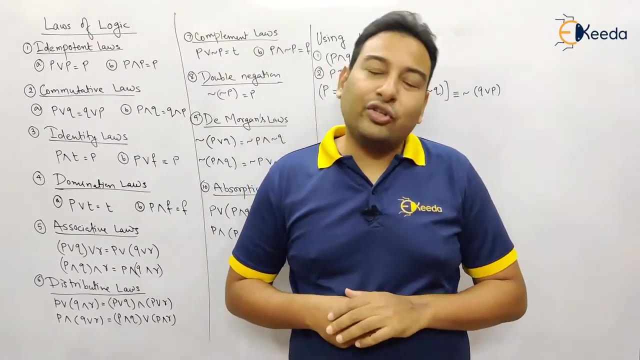 So better you remember the names. commutative laws. Commutative law means P or Q can be written as Q or P and the same goes with and that is P and Q is equal to Q and P. The next is identity law: Here and, and, or. Remember the truth table of and and or. What is the truth table? 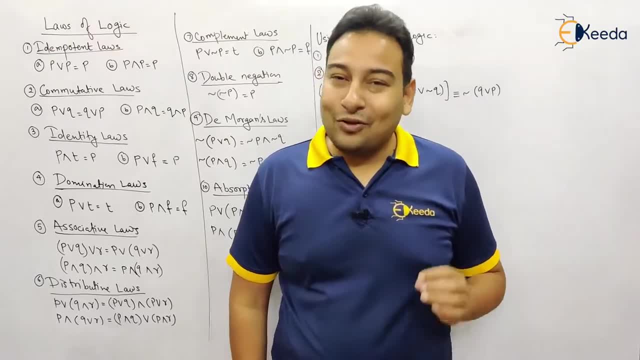 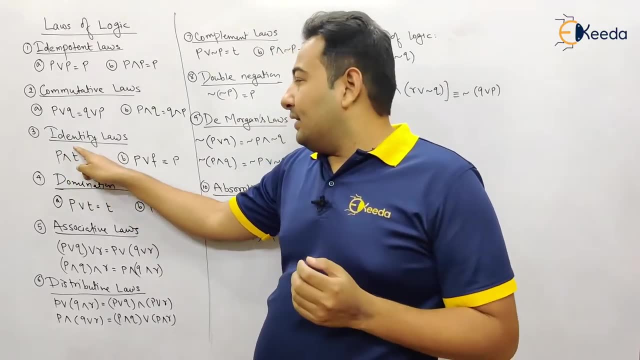 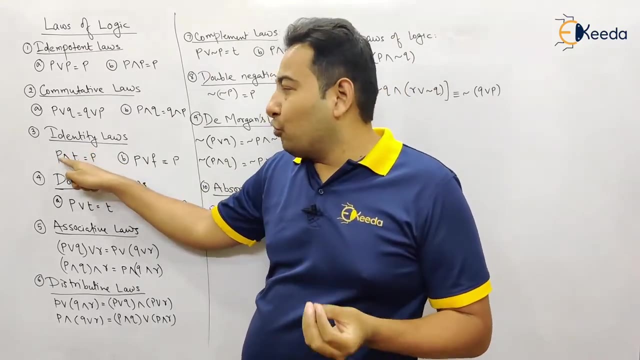 True and true is always true. False or false is always false. What does that mean? If both are true, the answer is true. See, here, this value is true. Now the result depends upon the value of P. If P is true, the final answer is true, because in that case both will become true. 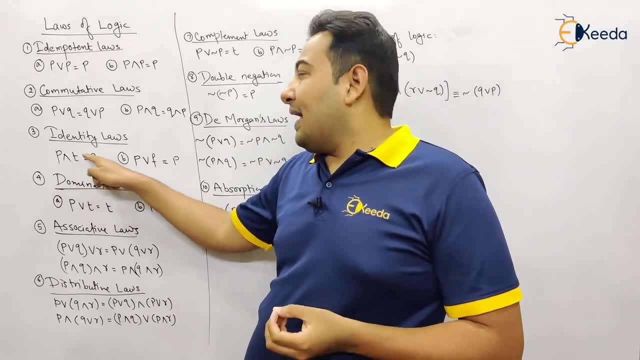 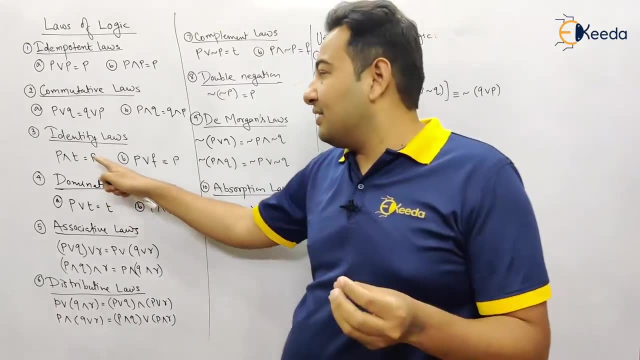 And if P is false, the answer will become false, because one will become false and the other will become true, And the condition is: both should be true for the answer to be true. That means this resultant is dependent on the value of P. Therefore, the result is P, The next is or. So the same logic. 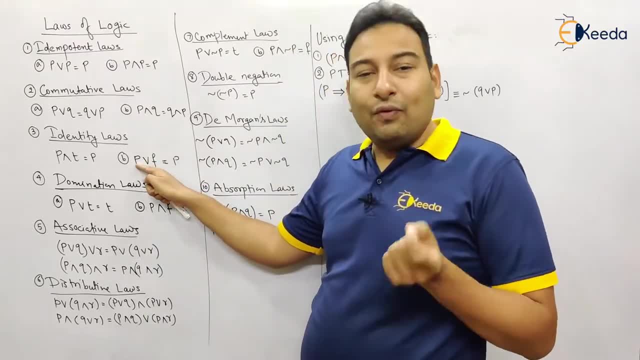 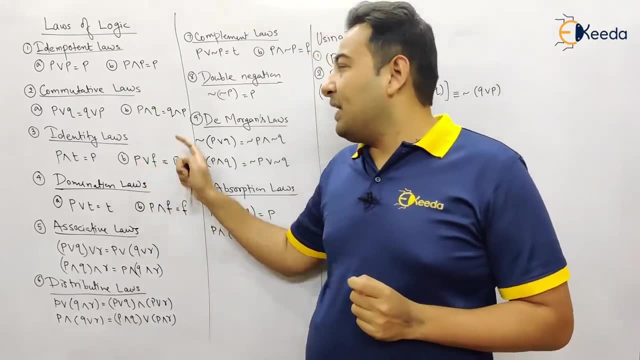 false or false is always false. This term is false. So, whatever is the value of P, that will be the result. If P is false, the answer is false. If P is true, the answer is true. Therefore, the answer is P, and these laws are called identity laws, Next domination laws. 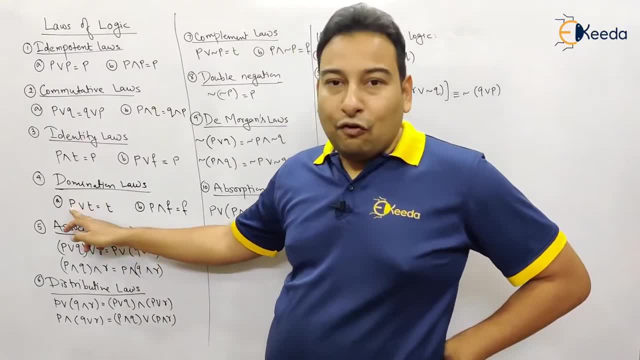 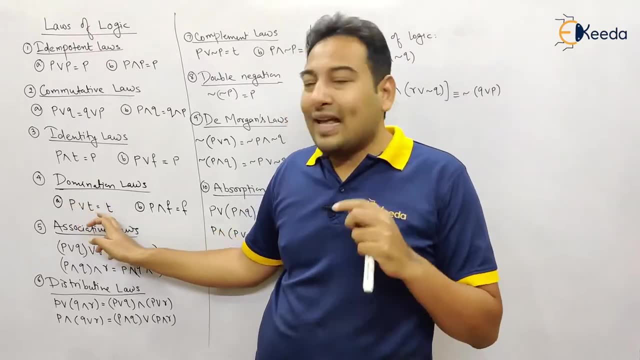 In the same logic. see here: whatever will be the value of P, the answer is true. Why? Because in case of or, both should be false to get false. If one is true, the answer is true, Whether P is true. 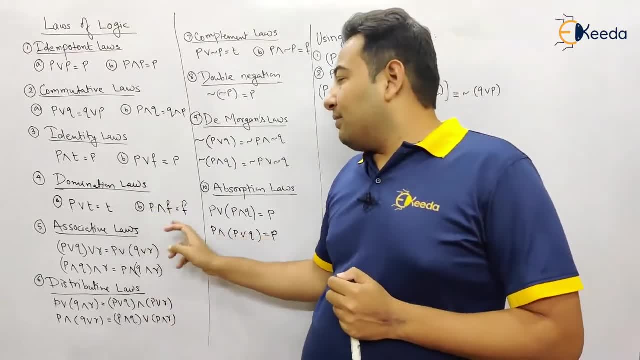 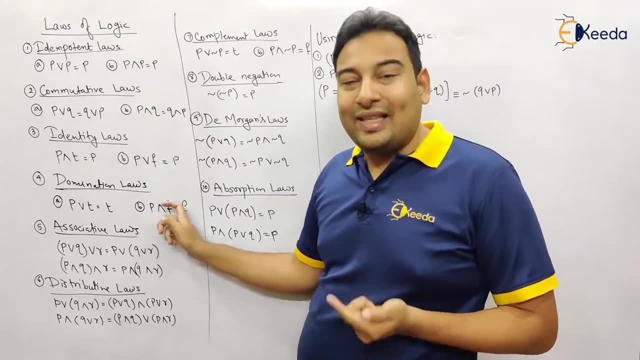 or false doesn't matter. Therefore it is called domination laws, And the same story is here. If both are true, then the answer is true, But here one is false. So whatever may be the value of P, the answer is false. So this is your domination laws. The next is associative and distributive. 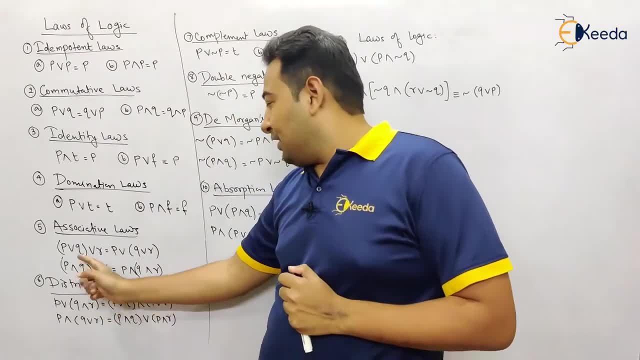 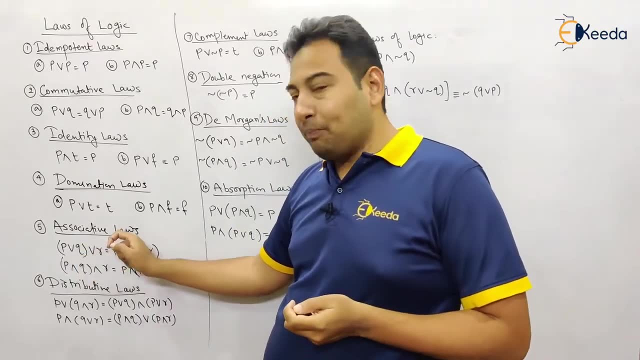 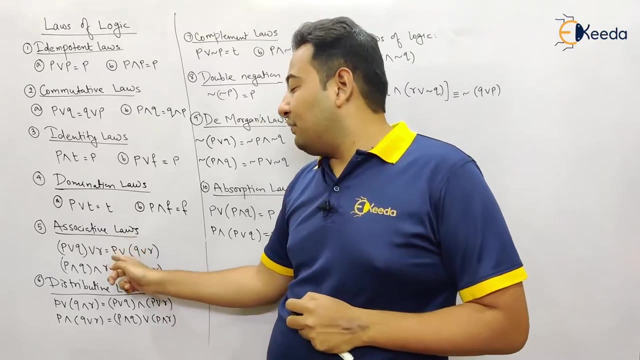 We are comfortable with that. Associative means you can shift the bracket- See, first you execute this and whatever is the result of this particular bracket will be evaluated with respect to this. Or you can shift this bracket First, you evaluate this and whatever is the result, evaluate with this. The answer is same, So that is your associative. 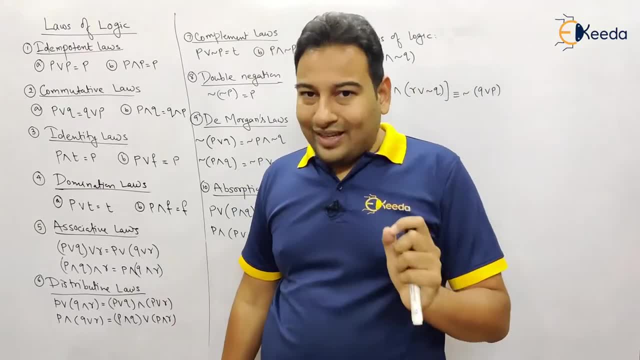 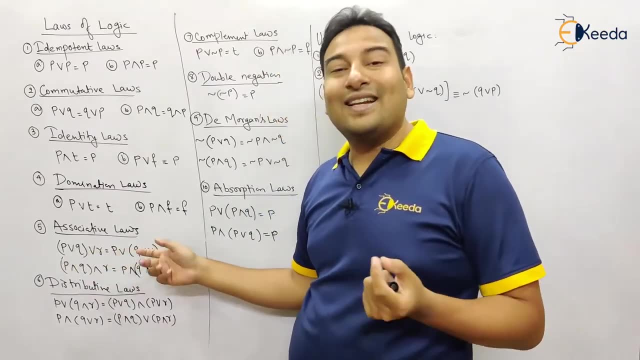 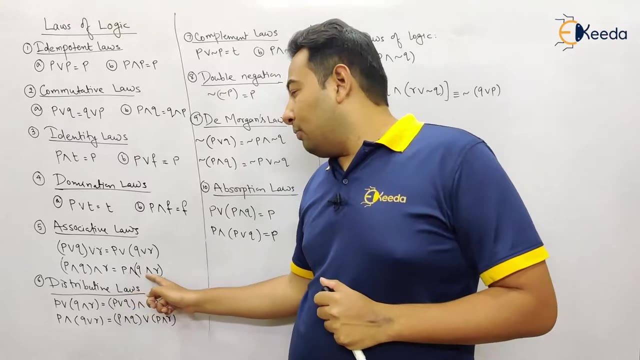 law And the important thing that you need to note here is: the operation is same, See throughout one expression. the operation is same, See all are, or, Or you can say disjunction, And the same law applies for conjunction, That is, and See here. If you observe this particular, 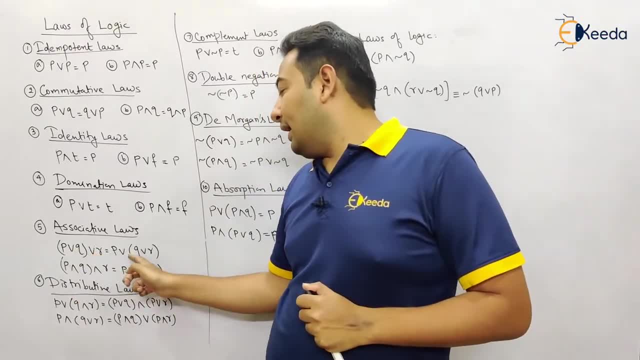 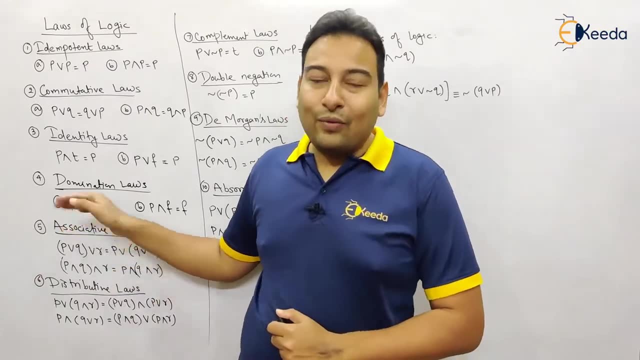 line all are and Here all are, or and here all are, and So this is your associative law, Next distributive law. Now, the difference between associative and distributive is: in case of distributive, the sign is different. In case of associative, see, the sign is same, But in case 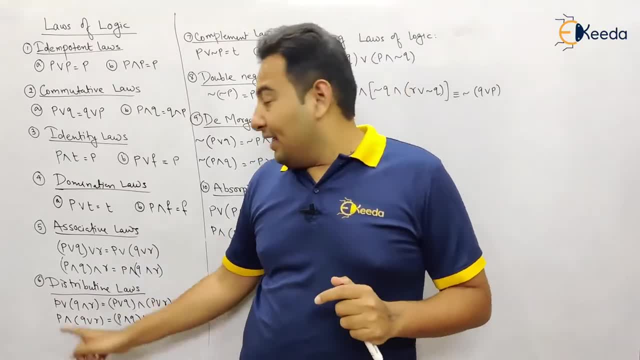 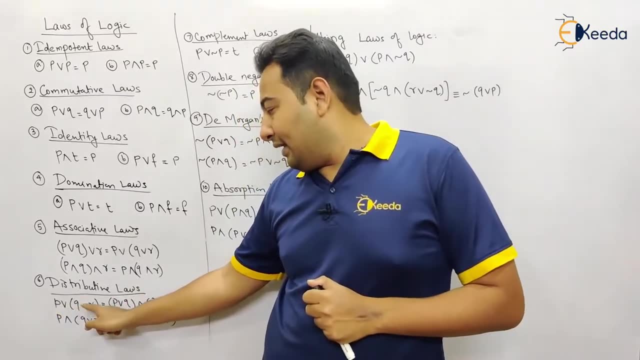 of distributive, see here or, and, and. The sign is different. If sign is same, associative law, sign is different Distributive law And what the law says- P or Q. this sign will come in between P or R And the. 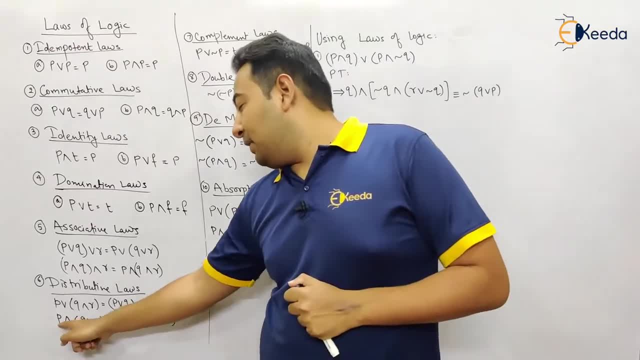 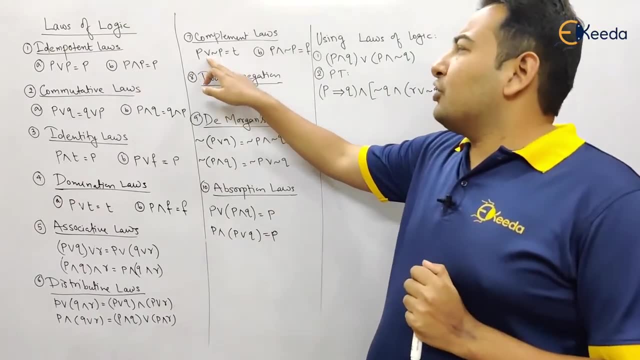 next is P and Q. This sign will come in between P and R. So this is your distributive law. Next, complement laws. Again, the same story, See this is, or. If this is true, this is false, Because 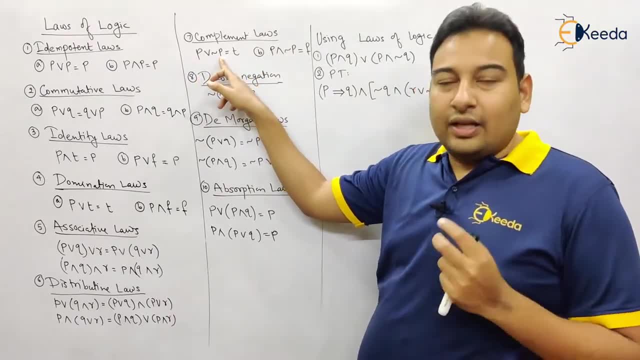 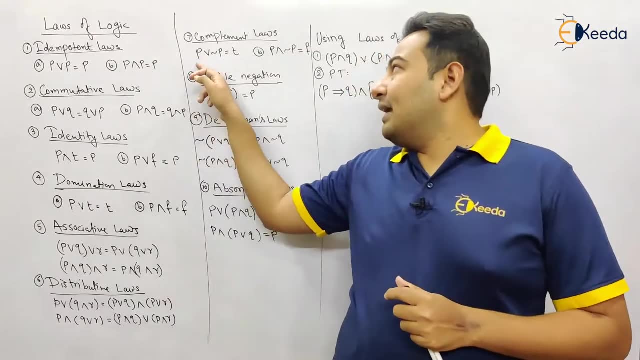 it's a complement. If it is false, then it is true. So, whatever may be the case, what will be false? it is false. So, obviously, if one is true, the other is false. If one is false, the other is. 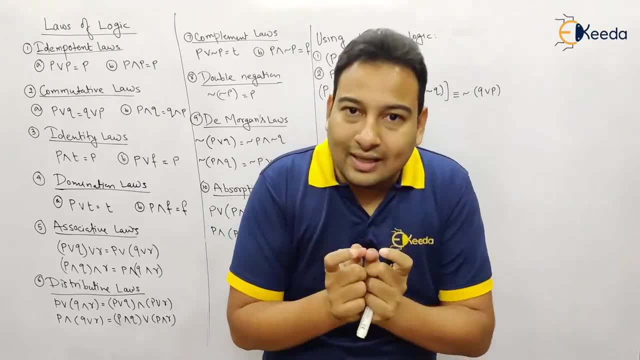 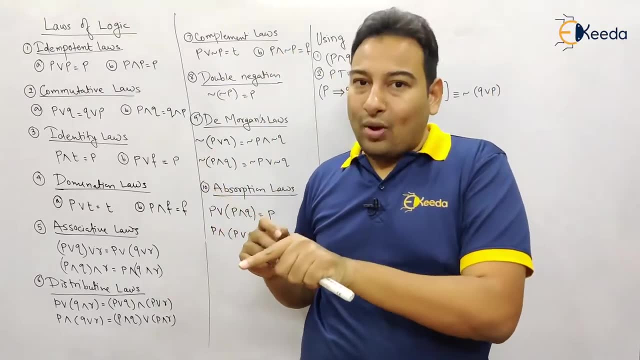 true. That means the answer can. we cannot get both false. That means the answer has to be true. And the same story here In case of: and we want both true to get the true answer, But here both can't be true. Therefore the answer will always be false. This is called complement laws. 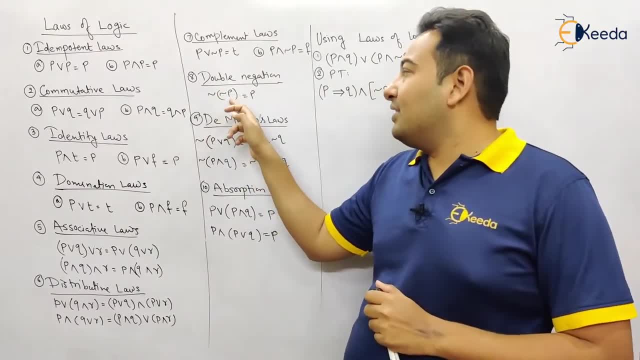 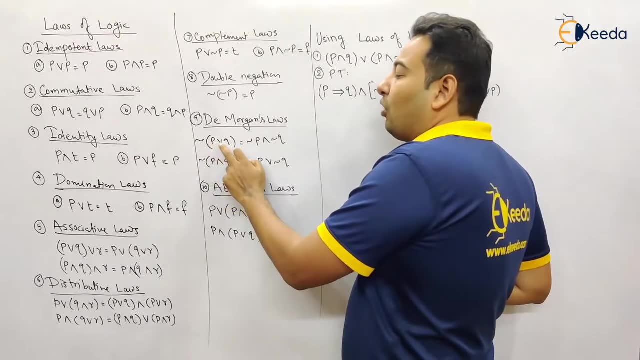 Double negation? very simple: If you have two negation, they will cancel each other and the result is P De Morgan's laws we already discussed. This is simply just open the bracket. negation P or will become and negation of Q. 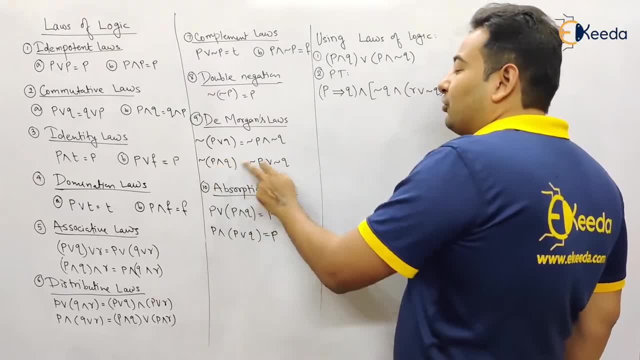 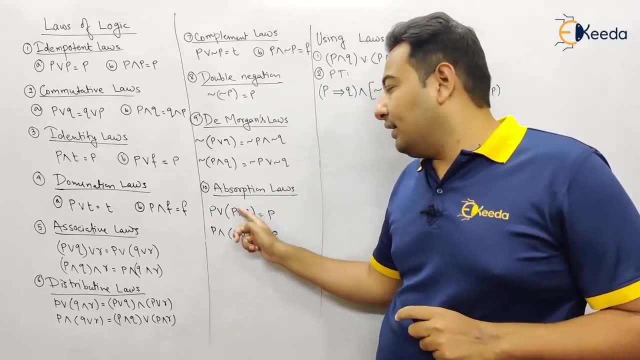 And here negation of P, this and will become, or negation of Q. And finally, absorption laws, very important law. See, here again you need to remember: sign should be different, Here it is, or here it is, and Here it is and here it is, or So sign should be different. And if you have 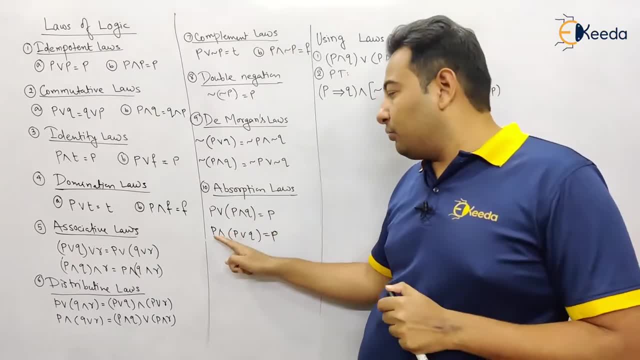 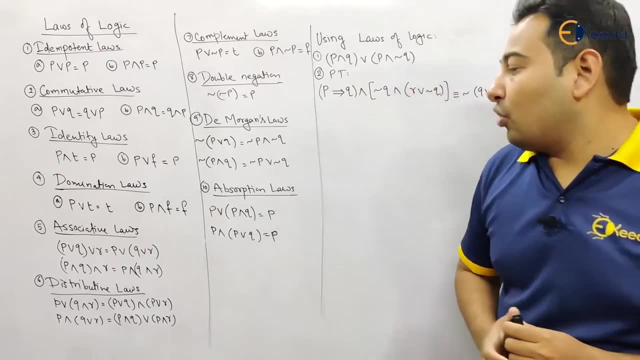 something like this: P or P and Q. And the second option is P and P or Q. So in that case result is P. So whatever is the repeated, that's your result. So this is called absorption loss. So these are the different laws of logic. So you: 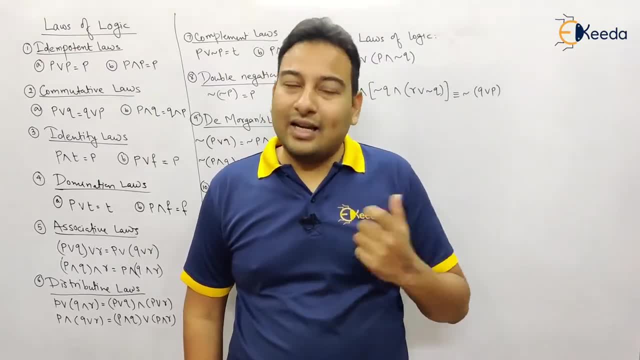 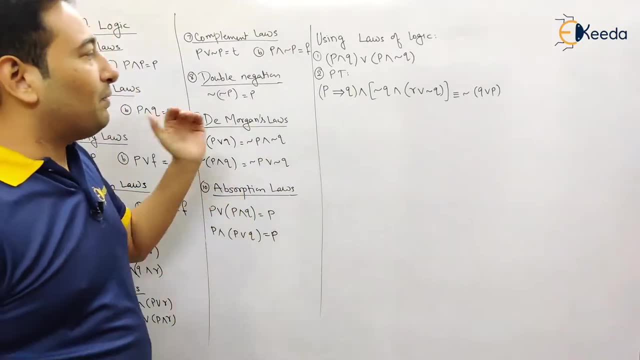 need to remember all the laws and, accordingly, you need to understand how to implement it, because you are very likely to get example based on this in the exam. So let us discuss two problems based on this law. The first problem is: we need to simplify this expression. So the first expression: 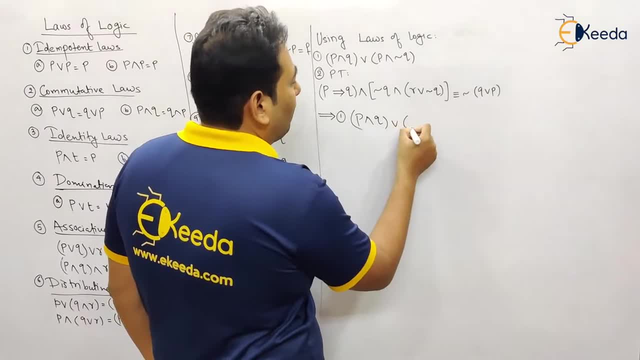 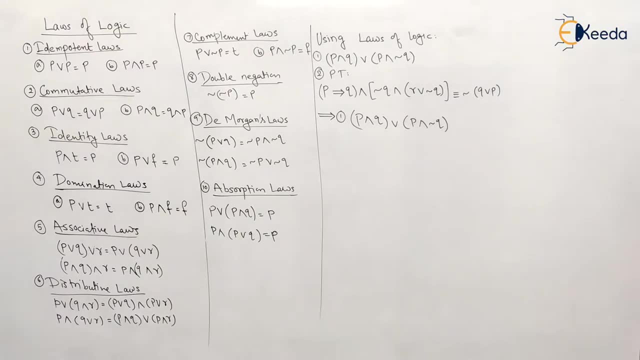 is P and Q or P and negation of Q. So this is the first expression we need to simplify. Now, if you observe, you can apply distributive law. See what is the distributive law. See here: this can be written in this format. Y-several size is also true. That means this can be written in: 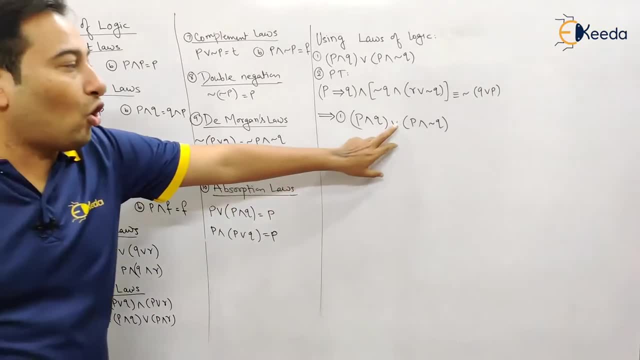 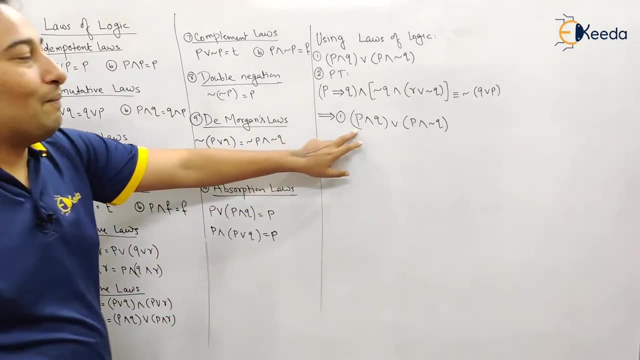 this particular format. If you observe this pattern, there is OR in between. That means this particular law Will be applied. So P and Q or P and R. See here: P and Q or P and R. So in short, you can say this: 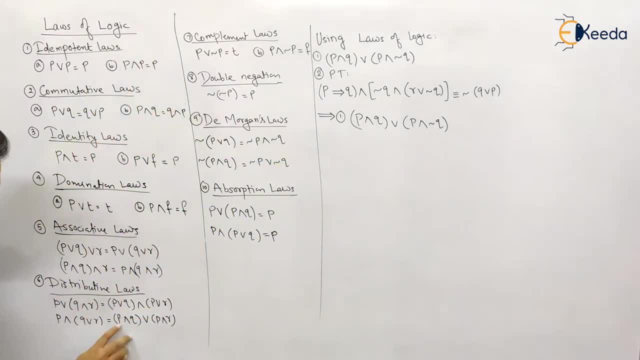 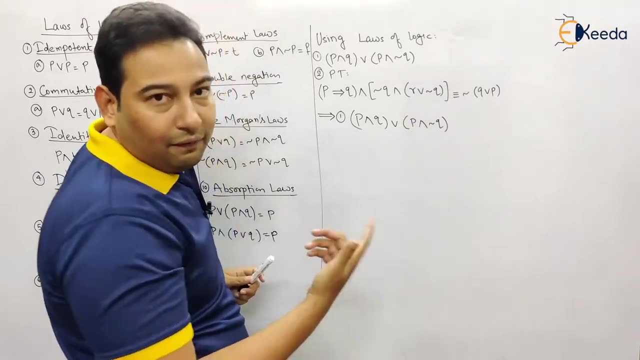 is Q and this is R. Obviously, both the terms are different. If you observe this pattern, this P is same, Here it is Q and R. So this is different And the same stories. here Q and negation of Q, They are different. That means you are going to apply distributive law and the law says P and 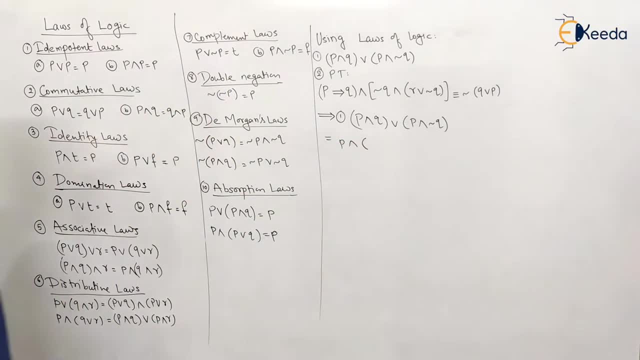 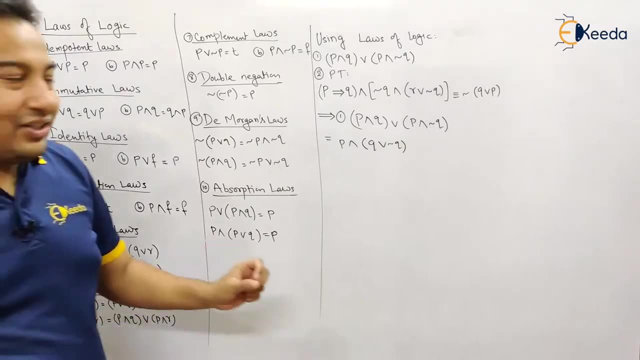 see here P and Q or R. So Q or R- Here R is simply negation of Q. So we applied distributive law On each step. you should mention the step, So which step you have used. So this is your distributive law. 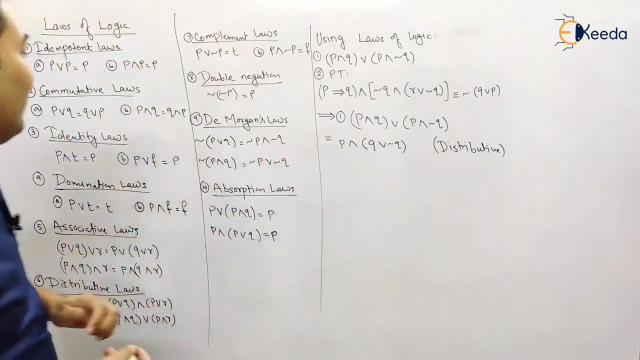 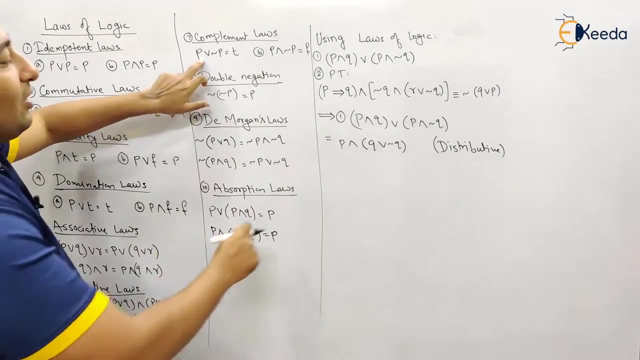 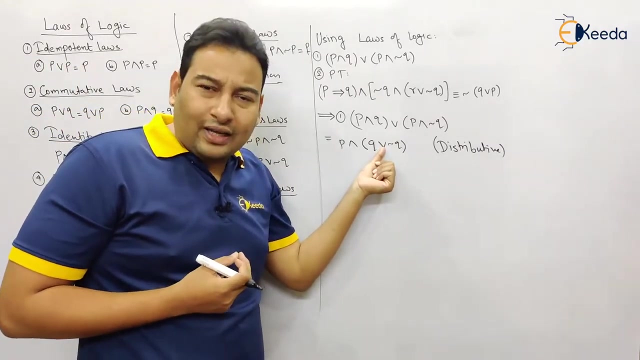 Next Now: Q or negation of Q. Now let us check which law we have for this. See here Compliment law. Q or negation of Q? The answer is true, Or you can calculate by yourself. See here: It is R For R's to be false. Both should be false, But they cannot be false at the 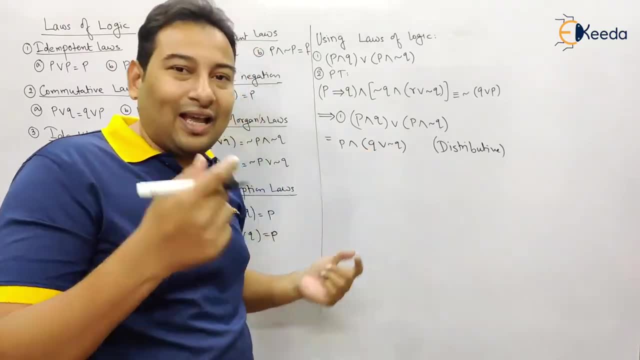 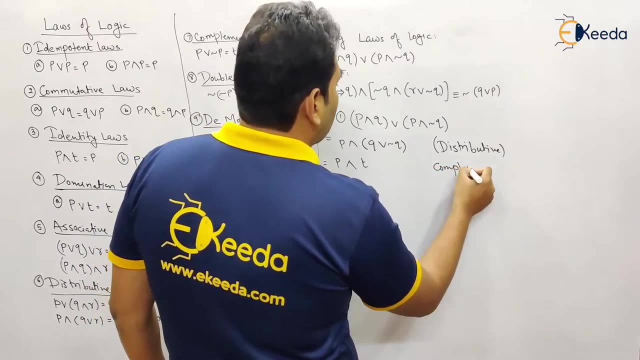 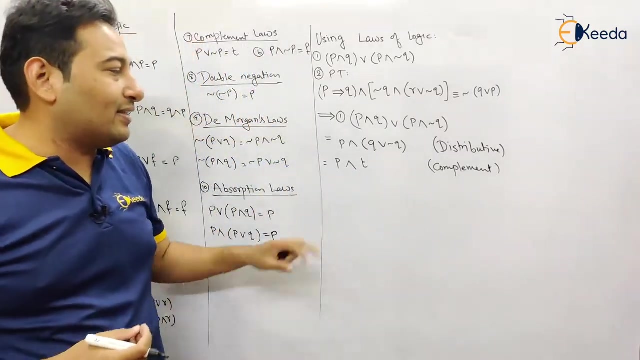 same time. So one will be false, The other will be true. That means this expression has must be true. So this is P and T. So we used compliment law. Next P and T: See without referring the law. If you know the logic, we can write it on the answer: See it's. 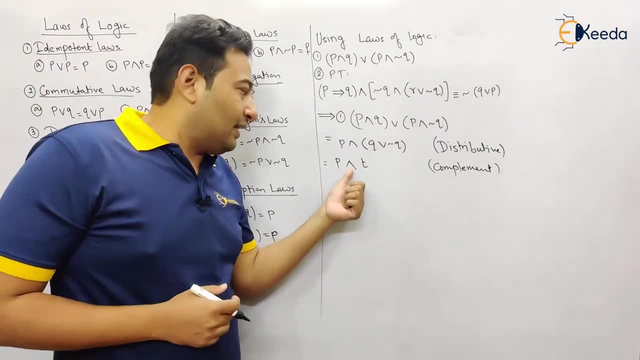 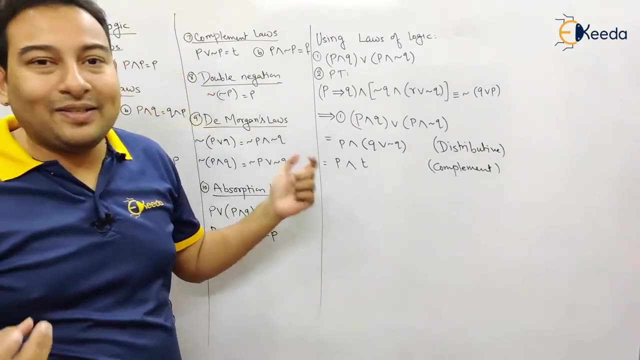 very simple: P and T, That means the answer will be true if both are true. so if it p is true, the answer is true. if p is false, the answer is false. that means the answer depends upon p. so, in short, we applied this particular formula, that is, identity loss. 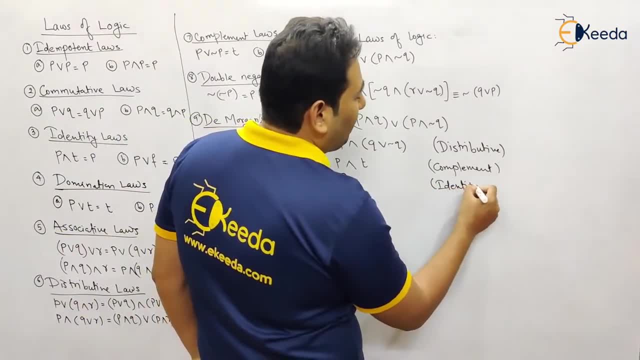 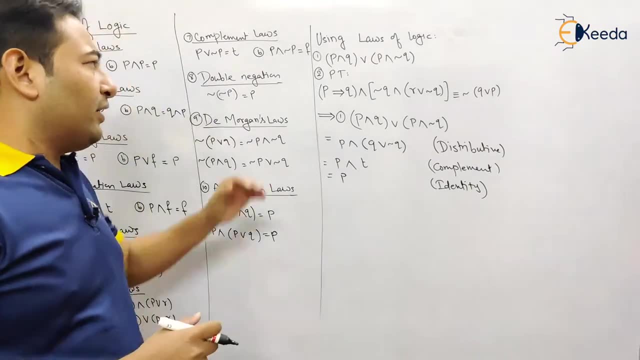 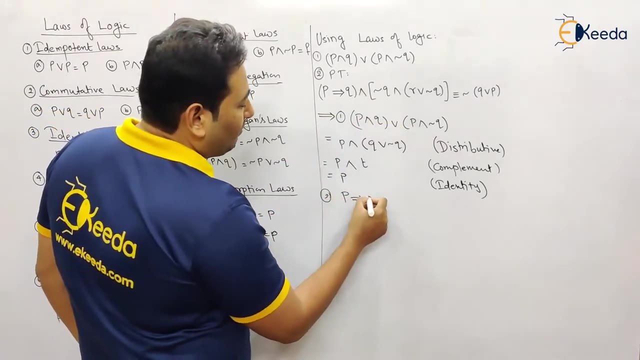 so this is what simplification is. now, if you don't remember the name, you cannot write it on this, so better, you need remember the name. so we're done with the first problem. let us discuss the next one. in the next problem, we need to prove this. so let us start with lhs. part p implies q. 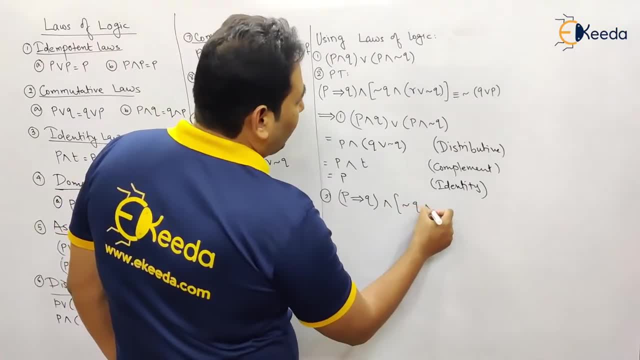 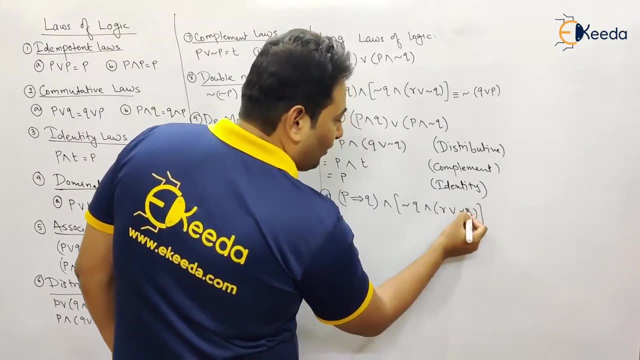 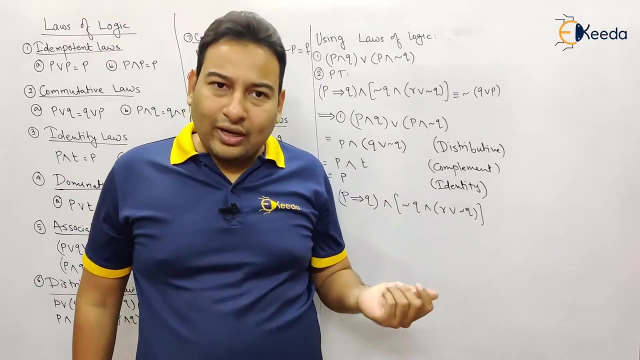 this is actually a logical equivalence. we have already proved logical equivalence with the help of truth tables, so truth table is also one method. this is another method, so it will be specified in the exam. if you nothing is given, obviously you can go ahead with the truth table method, that is. 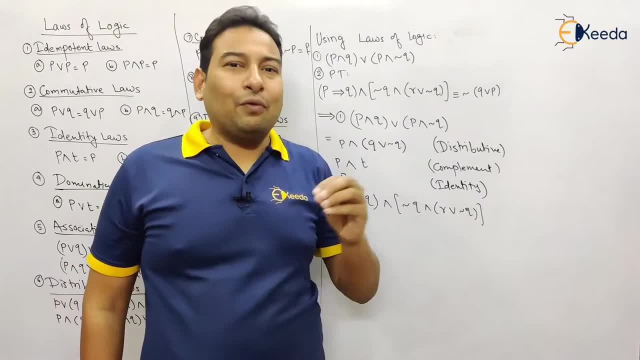 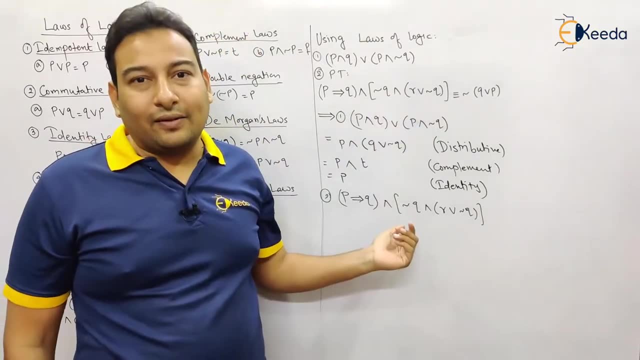 very simple and if you're comfortable with this, obviously you can go ahead with this, but whenever i've seen so many times, whenever this comes in the exam, it's clearly mentioned- use laws of logic to prove that if it is true, then you can go ahead with the truth table method and if it is false, 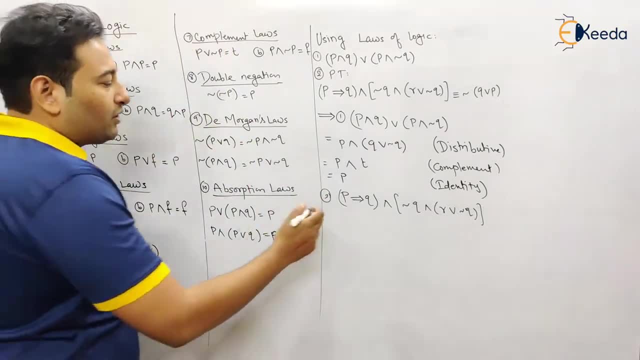 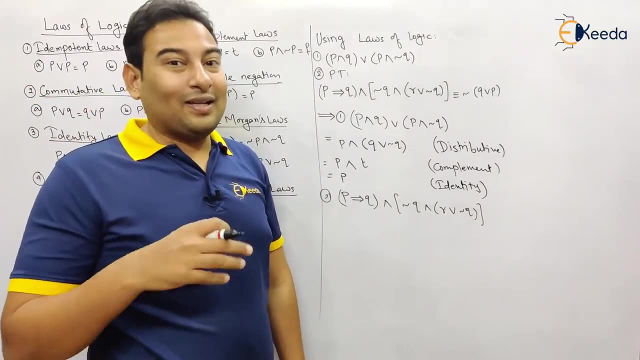 that is not given. obviously, you can use truth tables, so let's move on. first of all, p implies q. so what is the formula for p implies q. we have already seen this. formulas in converse, inverse, contrapositive: p implies q. you need to remember the formula, very important formula: negation of p. 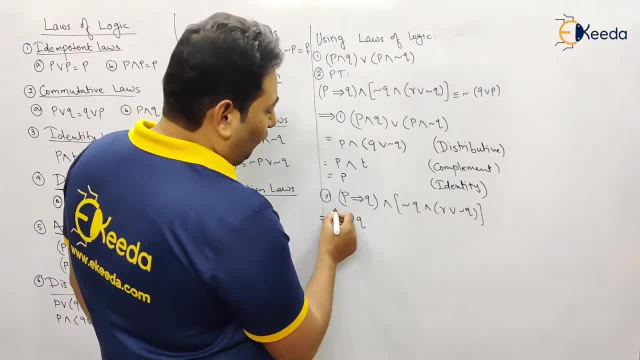 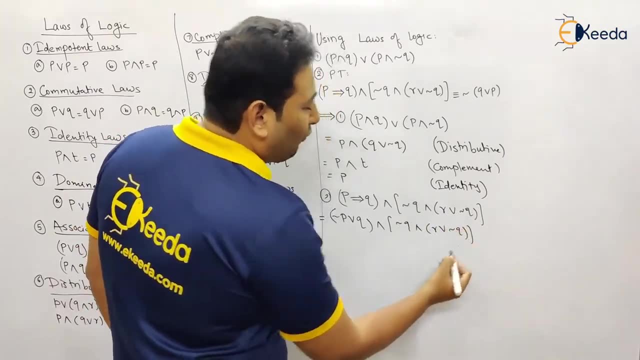 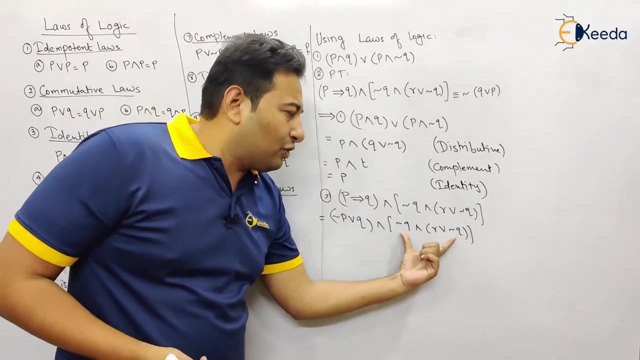 or q. so this is the formula and negation of q and r or negation of q. most number of times we're going to use distributive formula. but let us take which formula we're going to use. distributive formula is we're going to use here? first of all, focus on this particular term. can you see sign? 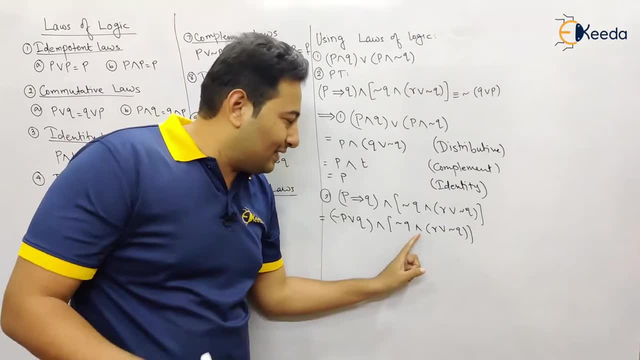 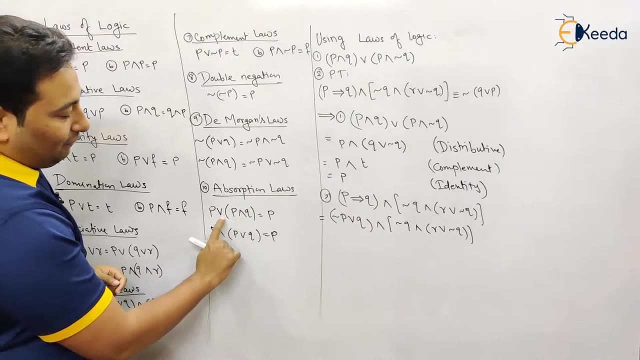 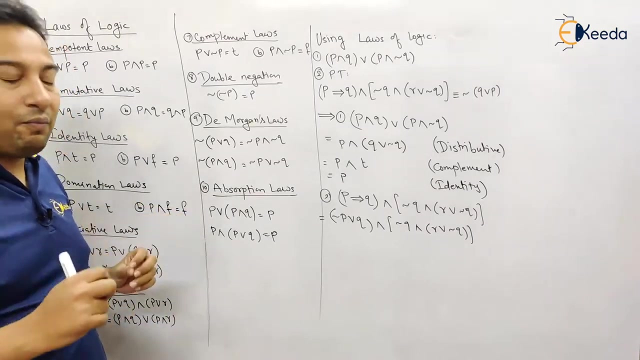 difference here and and or. there is a sign difference and the term is common. now let's move on. let's check what is absorption, absorption law? see, here the sign is different and one term is same. that means we can apply absorption law. but the problem is in case of absorption law, 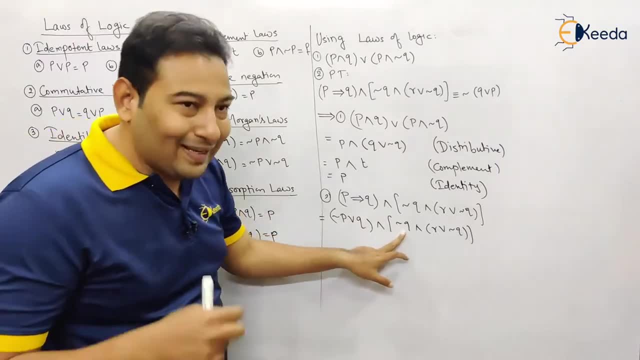 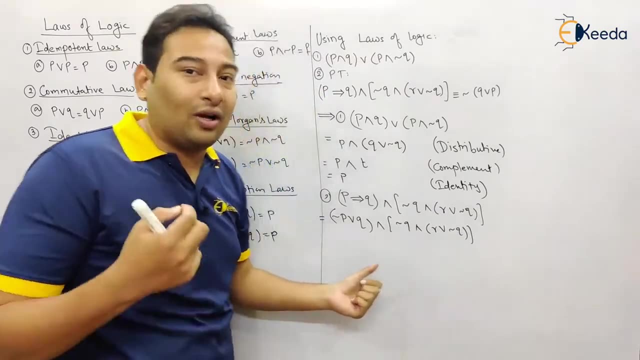 the first term should be same. that means if it is negation q here, here it has to be negation q. so can you make this term negation q or r? yes, we can do it. which law? commutative law. see what commutative law says: p or q can be written as q or p. so by commutative 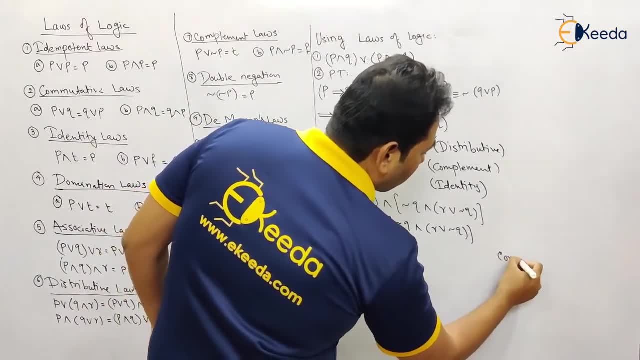 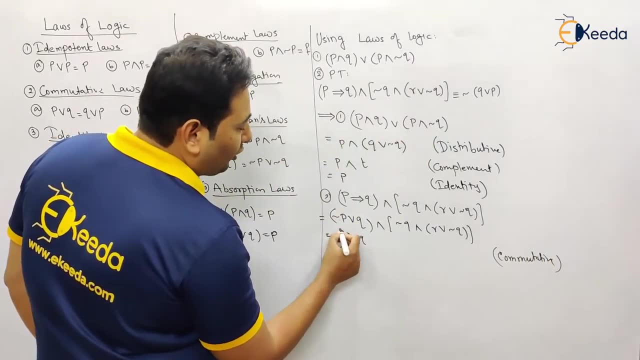 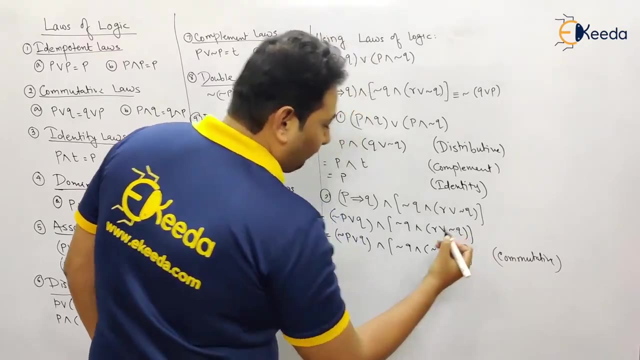 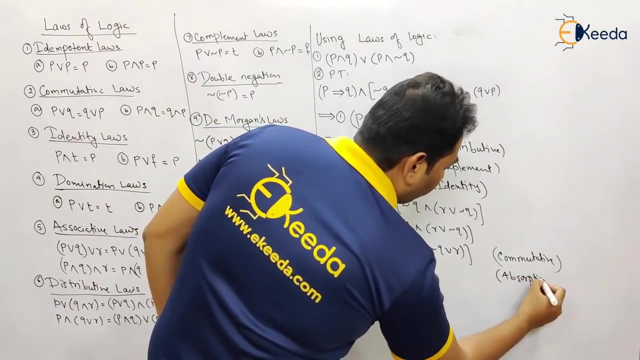 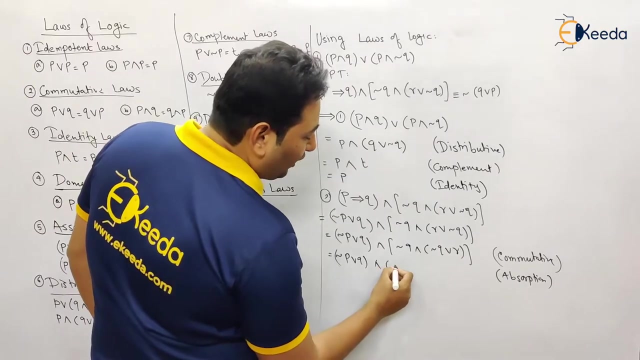 so what commutative law says? so this is negation of p or q and negation of q, and so this can be simply written as negation of q or r. now, by absorption law, this can be simply written as negation of p or q, and this will be equivalent to negation q. only see: 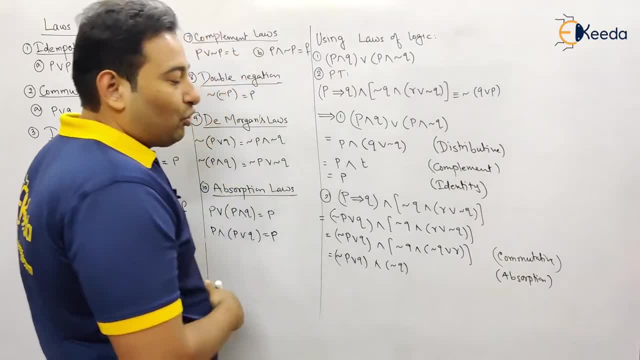 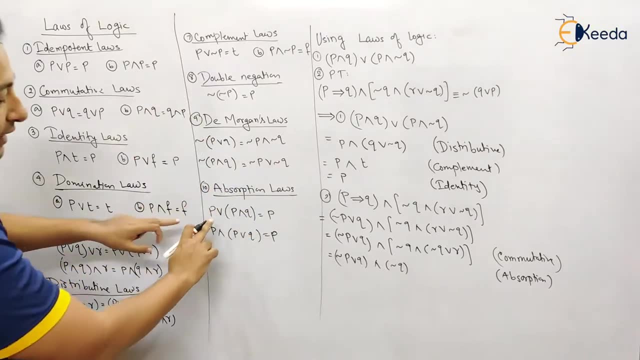 here. we applied the absorption law. what next? now we need to apply distributive law? see. in case of distributive law and absorption law, what is the difference? see the first. what is the thing common? sign should be different. see here. sign should be different. so this is the thing common, but in case of absorption law, two values. 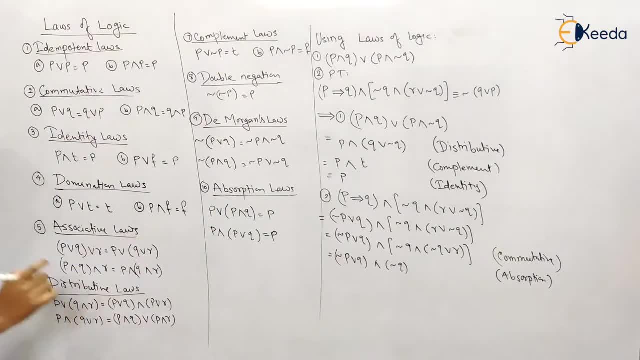 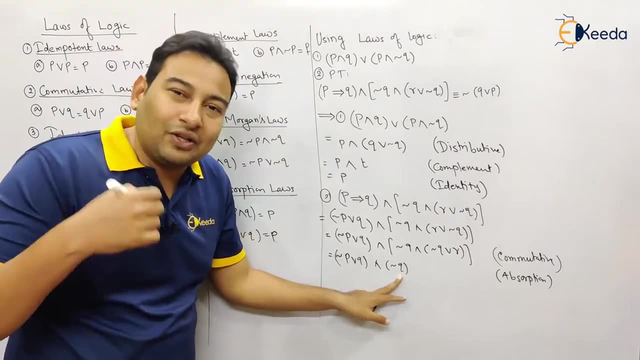 are same, but in case of distributive law all the values are a difference. so this is the difference between absorption law, distributive law. if you observe, here all the terms are different. that means no more absorption. this time we're going to apply distributive law because the 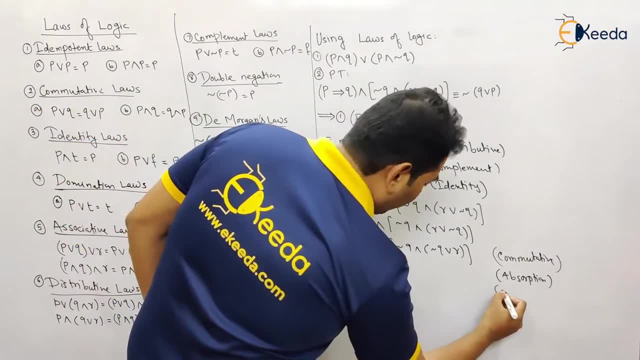 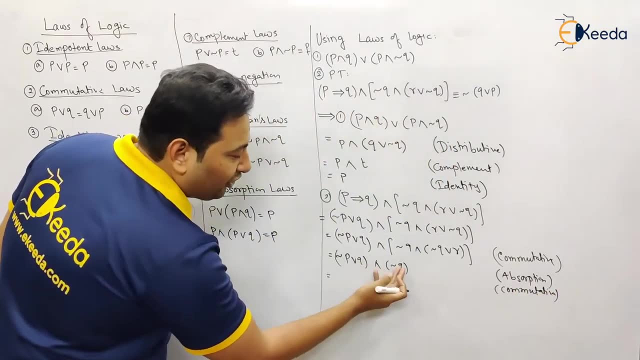 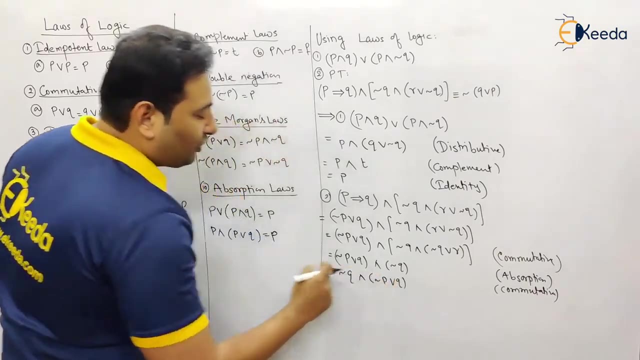 operations are also different. so first of all let us apply commutative. commutative so that will be comfortable with the form. you can directly apply distributive, no problem. commutative means this will come here and this will go that that side. so this is negation q and negation of p or q. now this is in the format of distribution law we can apply. 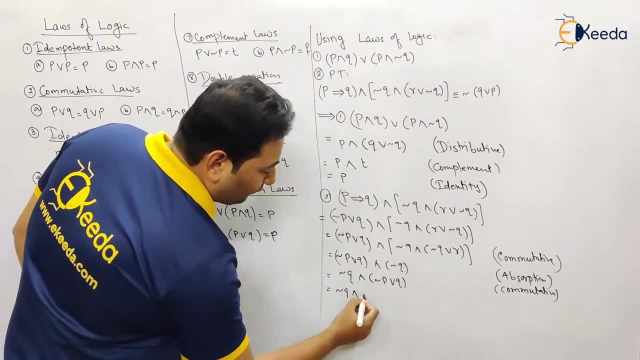 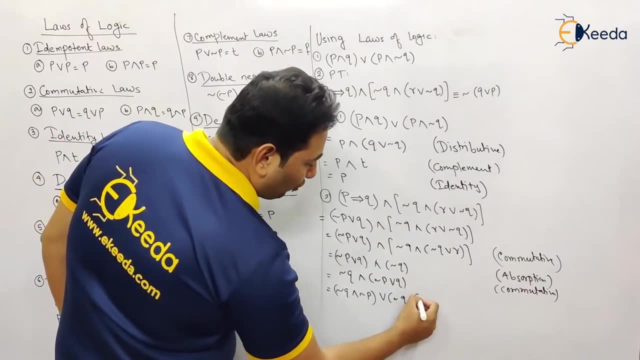 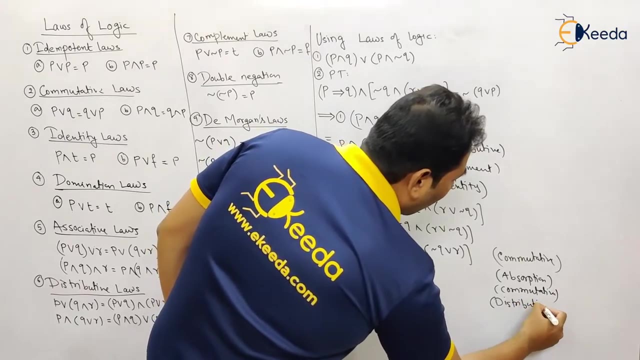 distribution law. so it's negation of q and negation of p, negation of q and negation p. this sign will come in between negation of q and q. so basically, this is your distribution law. what next now? it's very simple: negation of q and q. so, without referring the law by logic, you should 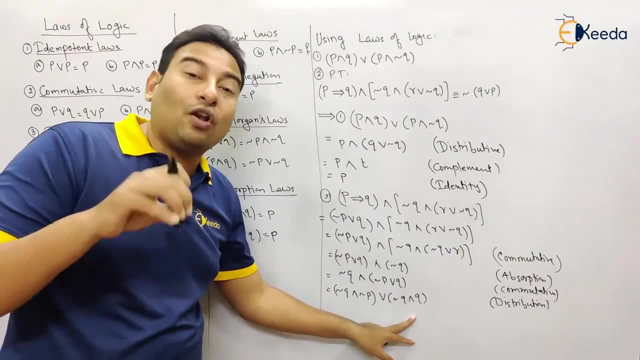 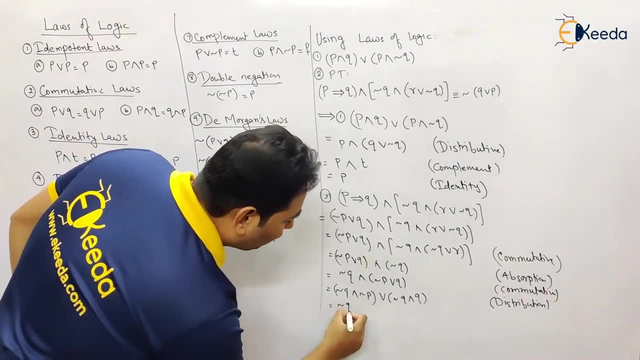 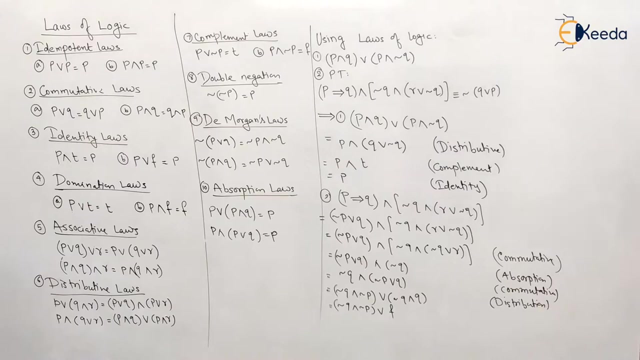 understand. see, if one is true, other is false. the answer will always be false because- and to be true, both should be true- that means this answer is false. so, in short, this will be negation of q or negation of p, or this is false. and this law, if you check, is this particular law.